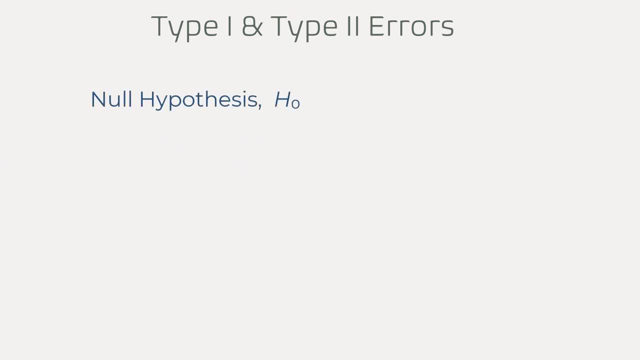 In hypothesis testing. the null hypothesis is a statement that suggests no difference or no significance, and it can either be true or false, And when making decisions, we either reject the null hypothesis or we fail to reject it. If the null hypothesis is true and we reject it, we have committed what we call a Type 1 error. 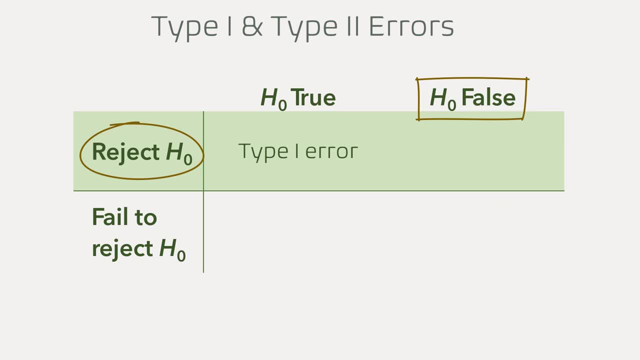 But if the null hypothesis is false and we reject it, we have made a correct decision. Similarly, failing to reject a true null hypothesis is a correct decision And failing to reject a false null hypothesis is called a Type 2 error. In other words, if the alternative hypothesis is true and we do not reject the null hypothesis, 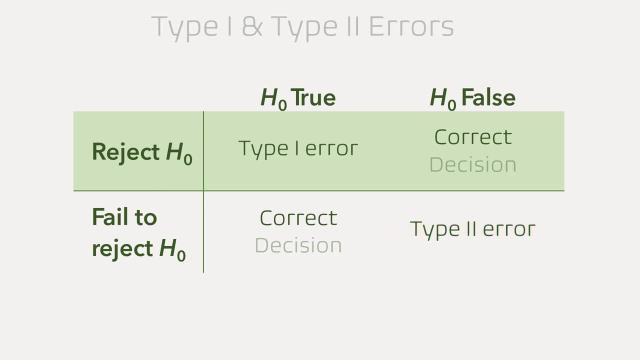 we have committed a Type 2 error. Type 1 error is also known as false positive, because we are saying that a result is significant when it is not, Or we are concluding that there is an effect Or a difference when there is not. 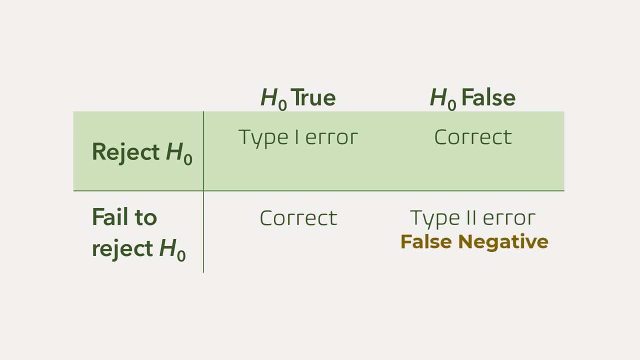 On the other hand, Type 2 error is also known as false negative, because we are concluding that there is no significance or no effect or no difference, when actually there is a difference. The probability of a Type 1 error is alpha, which is referred to as the significance level. 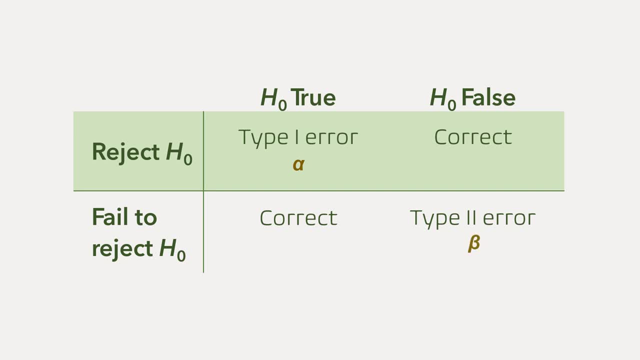 While the probability of a Type 2 error is called beta, The complement of beta is called power, Which is the probability of rejecting a false negative And not rejecting a true. null hypothesis is referred to as confidence. Consider this research question: Is the average driver's age different from 40?? 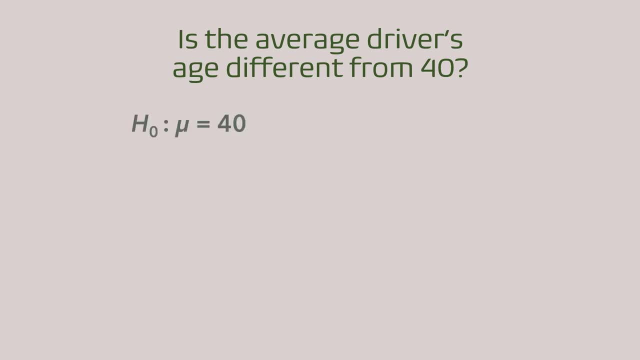 The null hypothesis here would be that the mean is 40 and the alternative would be that the mean is not 40. So what's the Type 1 error here? It would be rejecting a true null hypothesis. Rejecting the null hypothesis means that we are concluding that the average driver's age 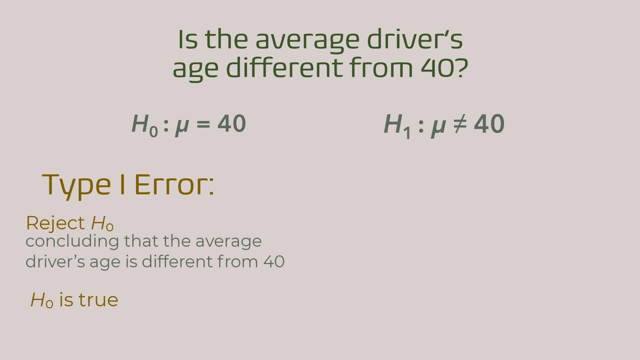 is different from 40. And the alternative would be that the mean is not 40. So what's the Type 1 error here Is the average driver's age is significantly different from 40. The null hypothesis is true means that the average age is indeed 40..